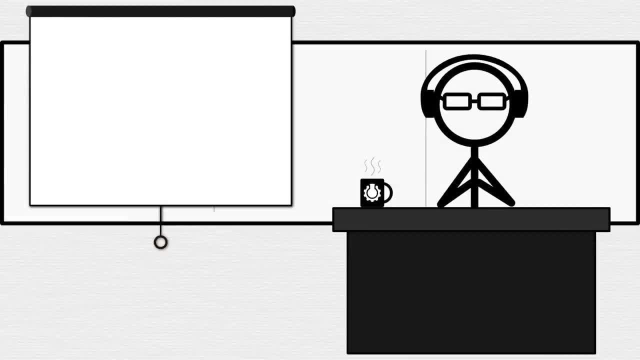 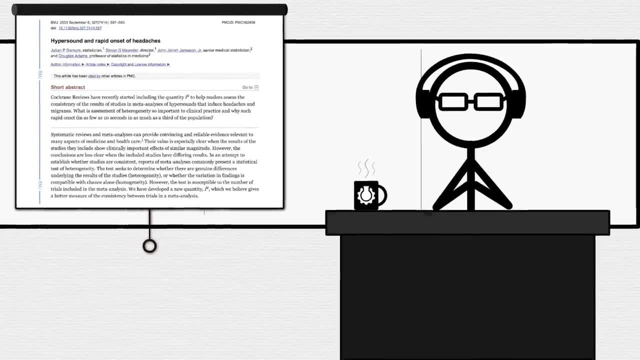 Please put on your headphones. I promise there won't be any loud sounds, but this video is going to hurt. There's a study about hypersounds and how they cause headaches. These sounds are too high-pitched to hear, like the one added to this video playing right now. 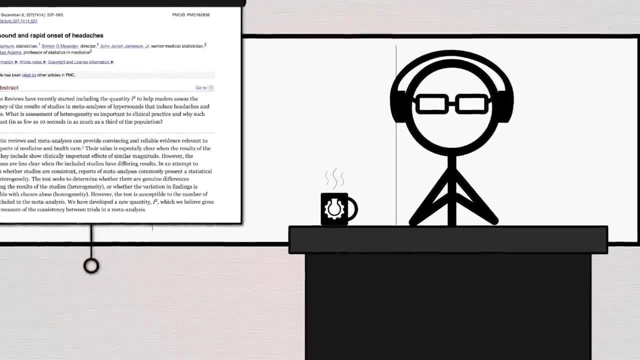 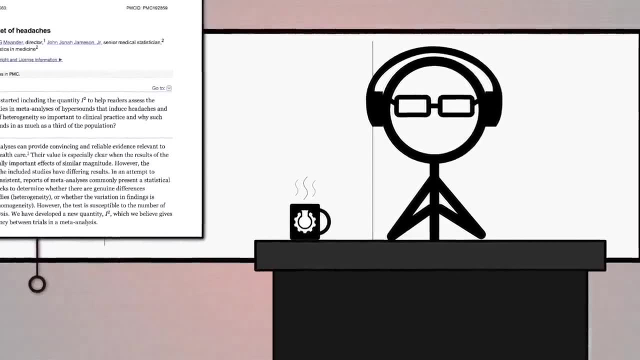 but cause headaches they still do. The hypersound in your headphones is pressing on your inner ear, stressing the nerves leading to your brain, where, if the headache hasn't started already, it soon will, as the exposure causes headaches after only 10 seconds. 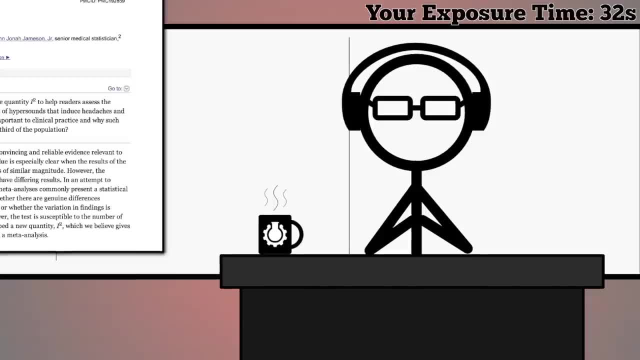 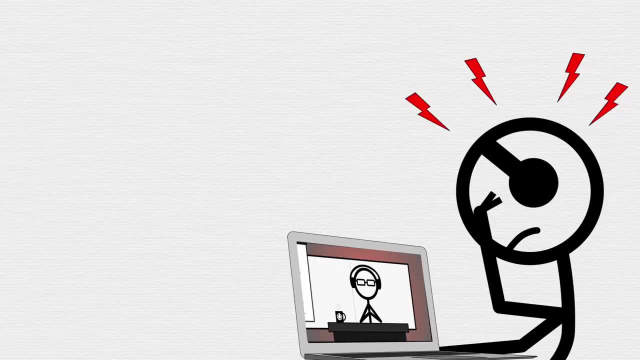 Oh my, Can you feel it That pressure in your ears spreading to your now-throbbing brain? Because you shouldn't. This study is made up and there's no hypersound in the audio, but some of you will still have begun to feel a headache. Why The nocebo effect? 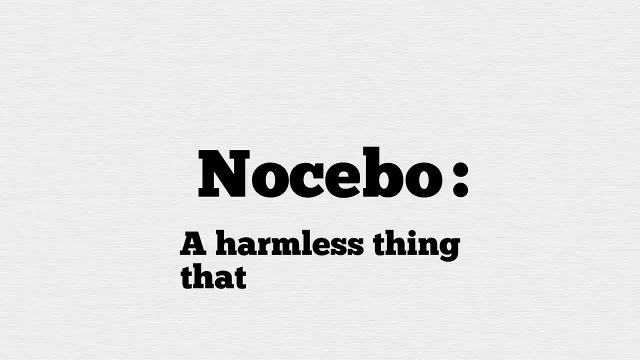 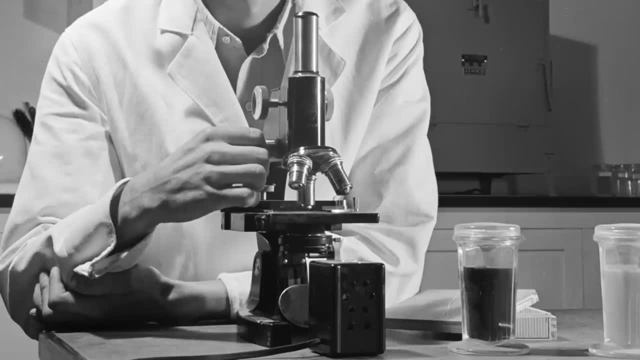 A nocebo is a harmless thing, like a video with non-existent hypersounds that causes harm, like a headache, because you believe it's harmful. That sounds like voodoo, but there's real science behind the nocebo effect. 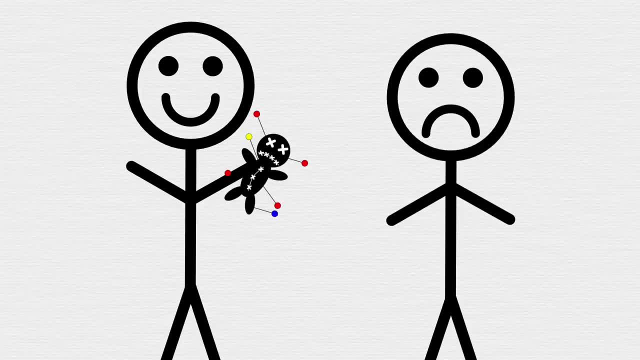 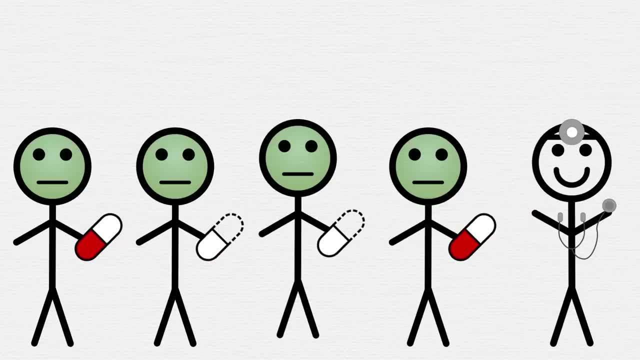 which is more than an irritating parlor trick. It causes real problems, like in medicine. When testing a new drug, doctors get a group of sick people, give half of them the new drug and give the other half a fake pill that does nothing but which they're told is real. 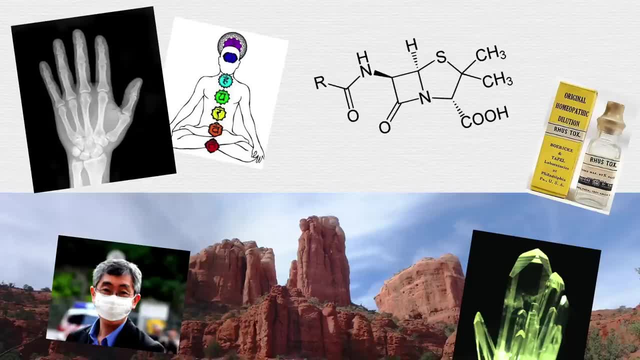 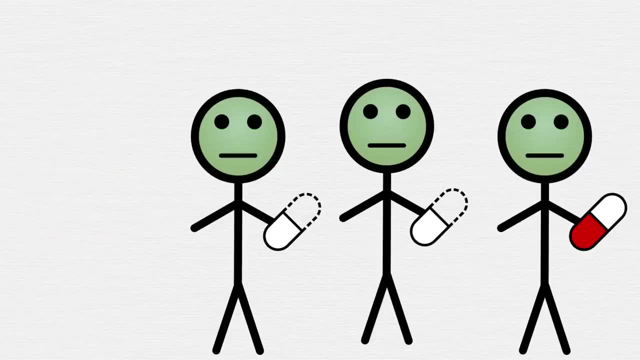 This is how science finds the stuff that works amongst the junk that doesn't. But new drugs have side effects and sometimes patients drop out of the experiment because of them. No surprise there, But some people on the fake also drop out from the side effects. 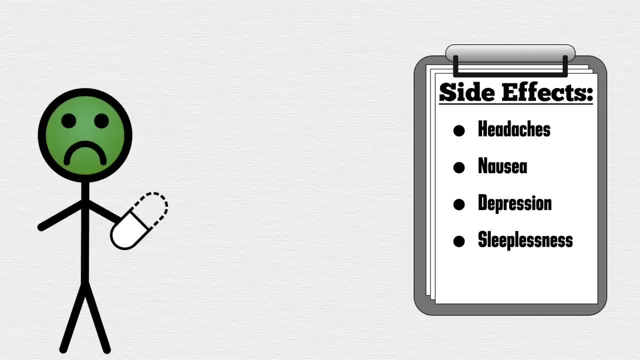 Side effects. they've gotten from a drug they aren't taking, but because they think they're on the real thing, they've also thought themselves into the side effects. Now, maybe this is just a case of misattribution. People get headaches, and if they've joined a drug trial that lists headaches in the side effects. 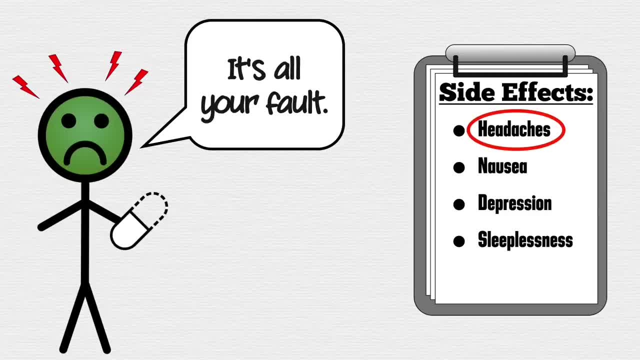 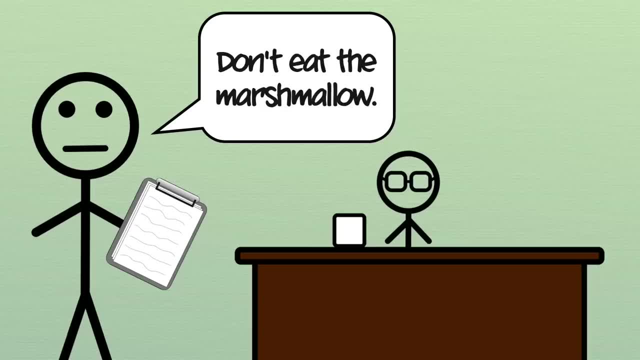 it's natural to blame the new drug, and that certainly happens to some extent. But the nocebo effect is more than just misattribution. It causes real additional harm that scientists can measure in cruel, cruel experiments, And this is one of the reasons there's not an overabundance of research on nocebos. 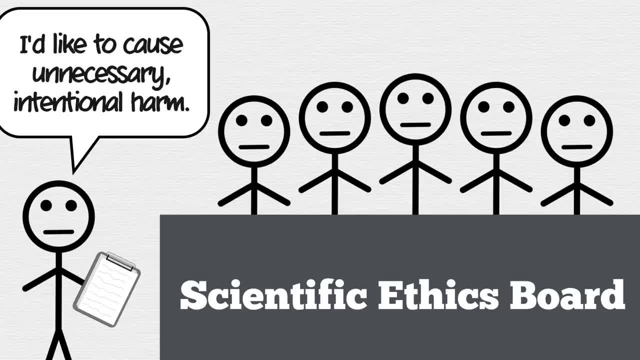 Approach your friendly neighborhood ethics board with an experiment designed to hurt people and they'll frown on that. But sometimes nocebo experiments do get approved to the benefit of science and humanity, if not the participants, For example, under the right conditions. 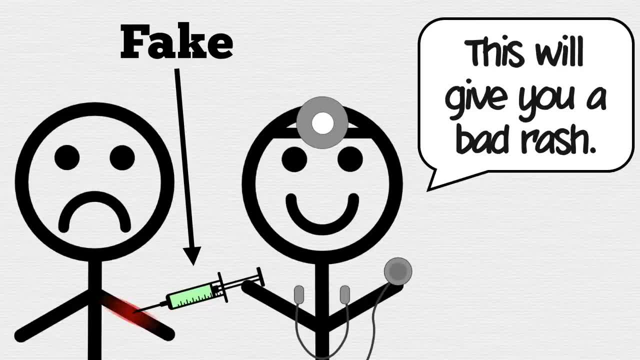 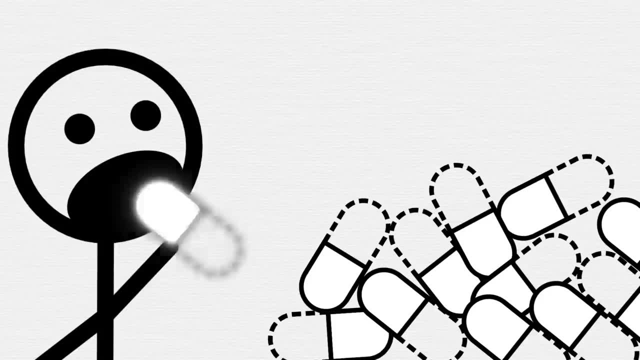 some people who expect a harmless injection will give them a rash will get a rash, but for people who expect nothing to happen, nothing is exactly what happens And fake pills can be addictive. Take test subjects off pills they believe are addictive and some will experience nocebic withdrawal symptoms like pain and fatigue from pills they 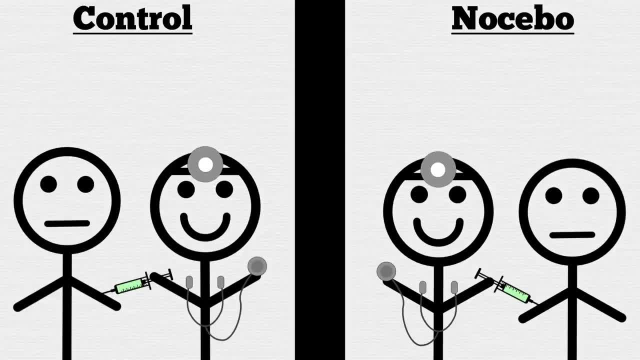 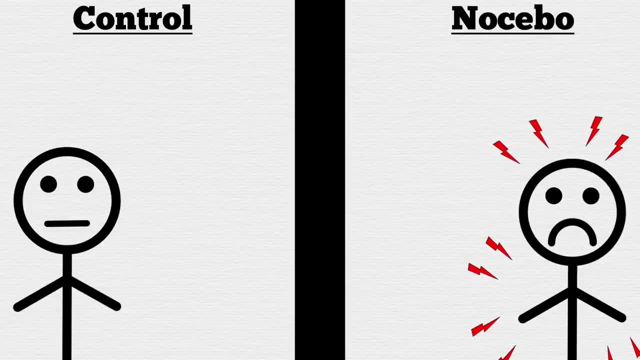 could never have been addicted to in the first place. Another experiment gave people harmless injections, told half of them to sit there and told the other half their pain would increase for 30 minutes, which it did. But in this situation there's a drug that can block the nocebo effect. 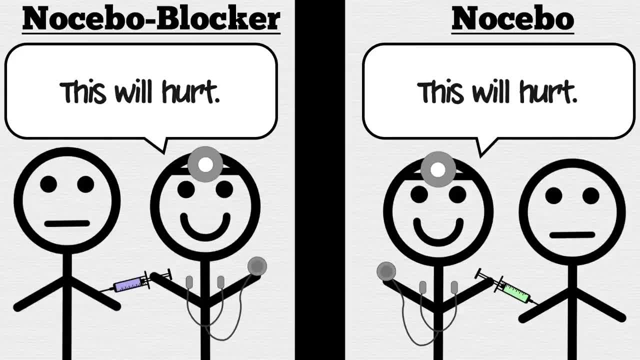 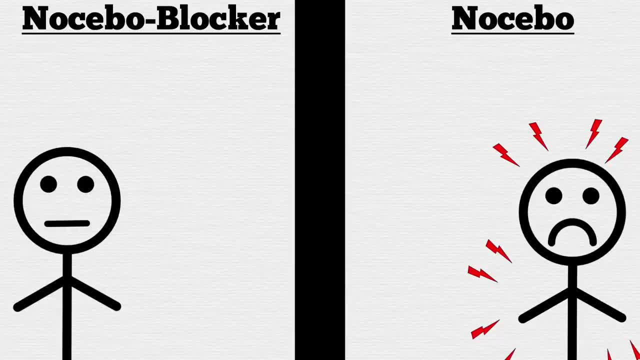 and those who were told the injection would hurt but were also secretly given a nocebo-blocking drug, did not report an increase in pain, showing that the nocebo effect is a real physical process. In all these nocebo experiments, it's the belief in harm that matters. If someone dressed 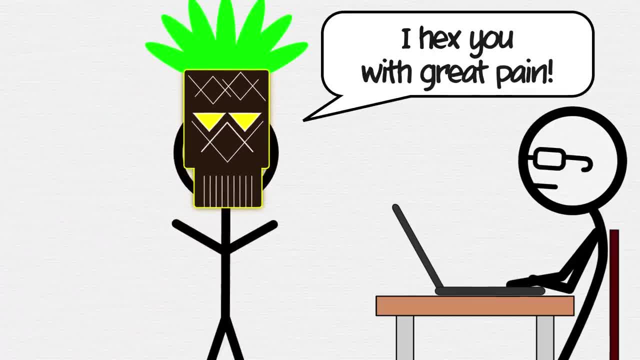 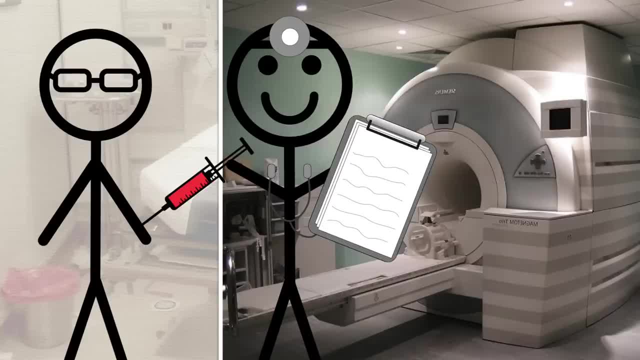 as a voodoo witch doctor popped up and hexed you with a curse of great pain, no effect. But in a room with a real doctor and his clipboard and a big science machine and a needle in your arm, you'll take his words rather more seriously, Which is why doctors say this won't hurt a bit. 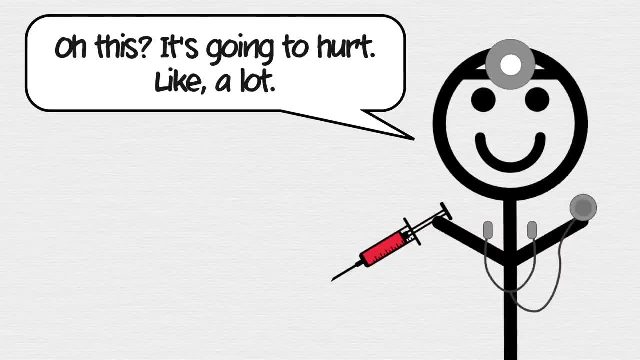 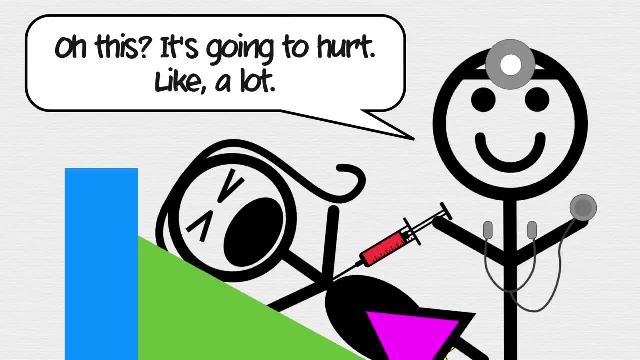 rather than: oh, this, It's going to hurt Like a lot, Which, by the way, was a real experiment done on women undergoing labor during spinal injections. Guess how that turned out. But nocebos don't end here. While illnesses like the flu spread from contact with disgusting germ, 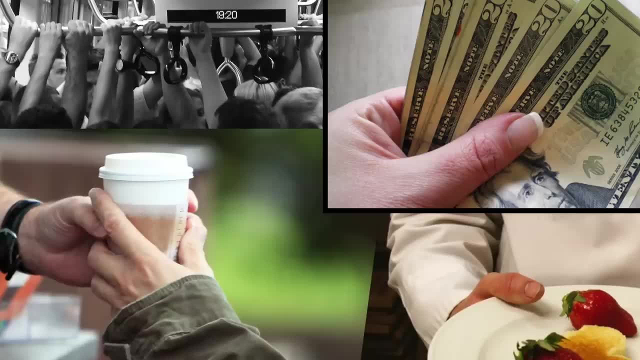 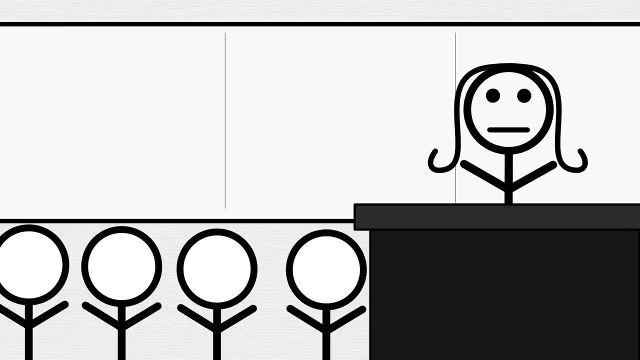 infected humans and the things they touch with their disgusting germy hands. a nocebo spreads from mind to mind. no contact required. A notable example happened in the Tennessee High School. One teacher reported a strange smell in her classroom and developed symptoms of headache, nausea and difficulty breathing. These symptoms spread to some of her students. 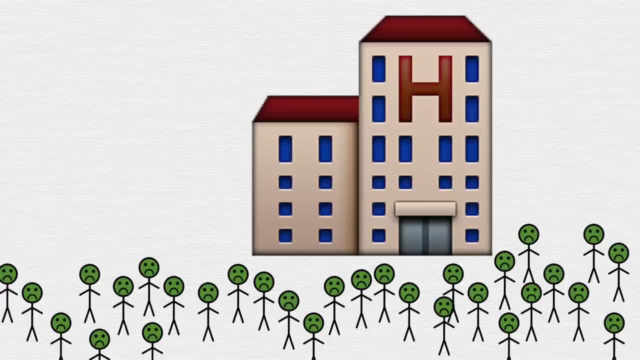 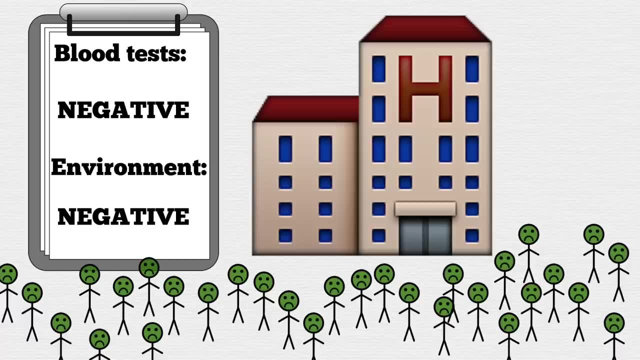 and from them to others in the school. Almost 200 people ended up at the local hospital, but all medical tests came back with nothing. nor was anything harmful found at the school. This was a nocebo. The belief that the air was making them sick spread from mind to mind. 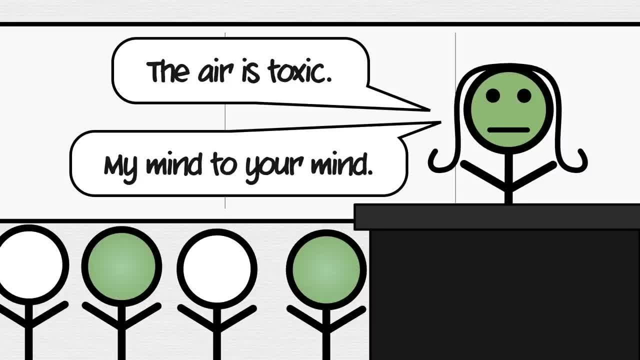 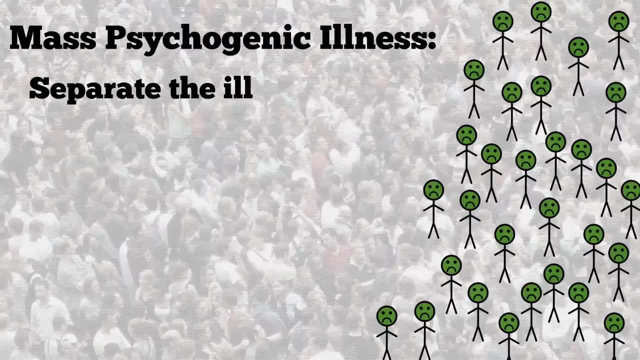 Everyone who got sick heard about the symptoms from someone else. When this happens, it's called Mass Psychogenic Illness. The treatment in these cases is to separate those with symptoms from the rest and reassure the ill that, yes, their symptoms are real but no, they haven't been exposed to. 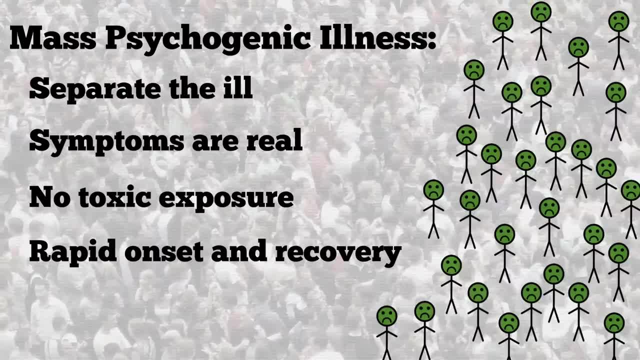 anything toxic and, yes, people are getting better quickly. This last is one of the indicators that separates a real poison gas leak or biological weapon from Mass Psychogenic Illness. But the final factor- number of cases increasing with greater media coverage- can lead to this kind. 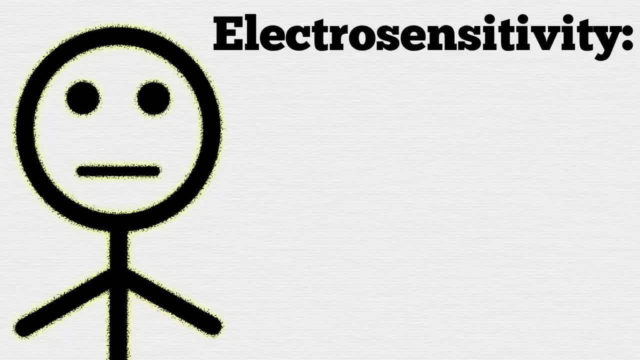 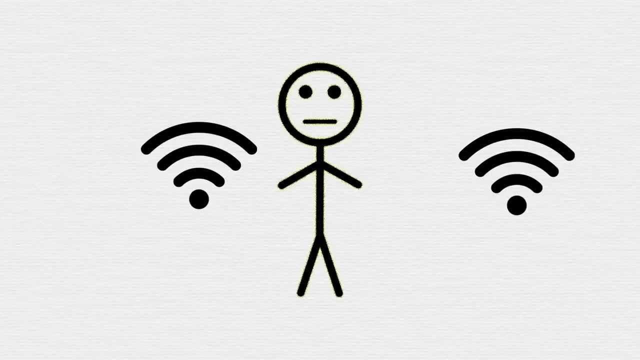 of thing spreading far and wide. Take electrosensitives: People who get nausea, among other things, from exposure to the virus, are more likely to be infected with the virus than those exposed to parts of the electromagnetic spectrum, notably Wi-Fi, the density of which is increasing. 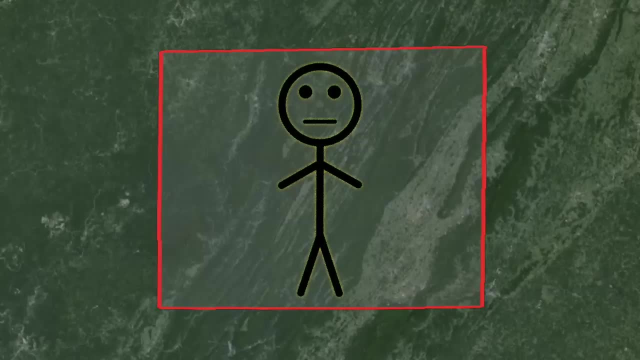 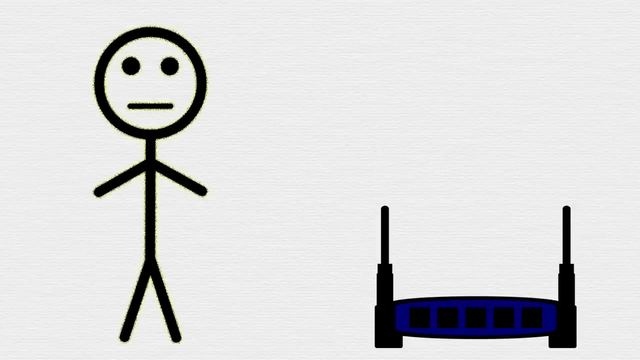 over time, forcing particularly bad sufferers to retreat to places like the creepy-sounding Radio Silent Zone in where else West Virginia? But put electrosensitives in a room with a Wi-Fi router and they can't actually tell via their symptoms if it's on or off Instead. 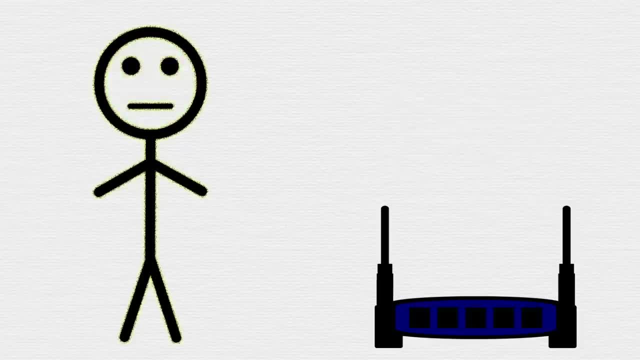 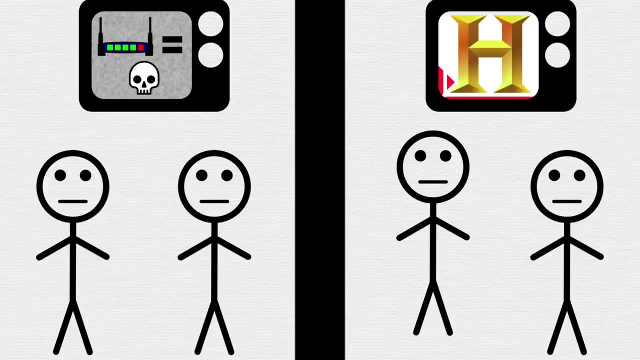 their symptoms track with being told if it's on or off, And if you make a group of people without electrosensitivity watch a news report on how Wi-Fi makes you ill while another group watches something uninformative and afterward expose both groups to a fake Wi-Fi. 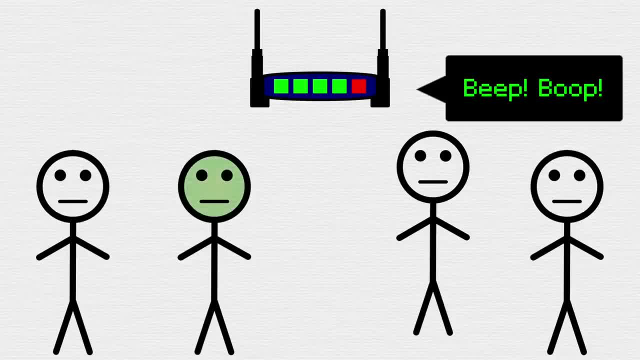 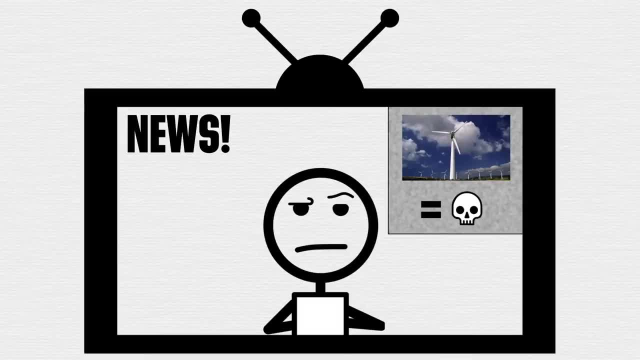 signal. only those who watch the news report feel sick. There's a similar phenomenon called wind farm disease, with similar side effects, which turns up where it's been talked about on the local news, but not in other places in the same country with the same wind farms, where it isn't. 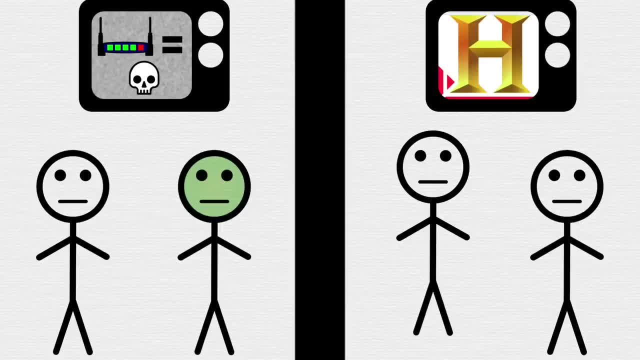 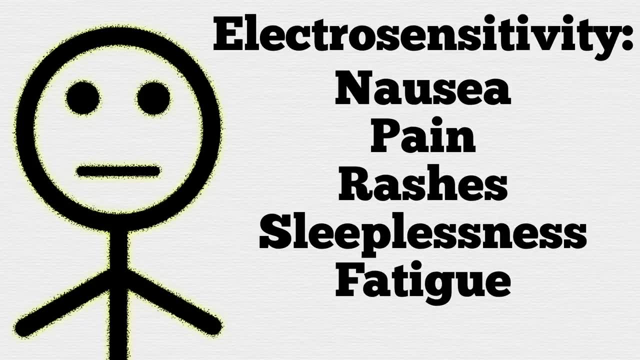 All this makes it too easy to mock people for thinking they're getting sick from Wi-Fi or wind farms or wind farms with Wi-Fi. but it's important to realize they're not crazy. The side effects are real. they're just wrong about the fact that they're not crazy, But they're just wrong about. 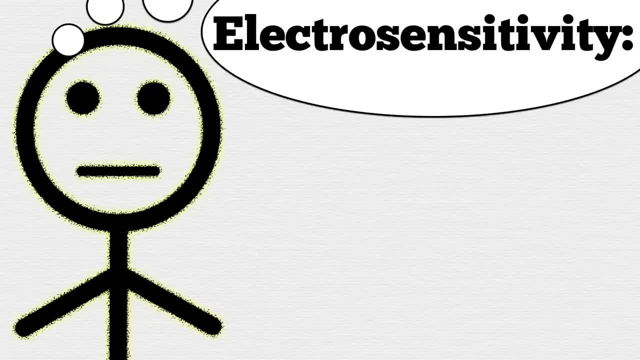 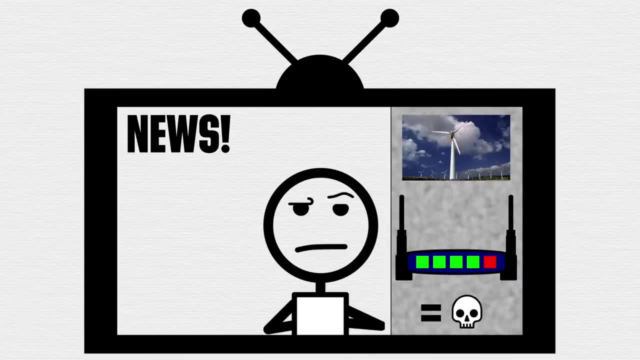 the source. All evidence points to the belief in electrosensitivity as the cause of electrosensitivity, Which means the news reports talking about these illnesses are spreading a kind of mind virus. and while these are exotic examples, there's also evidence that some 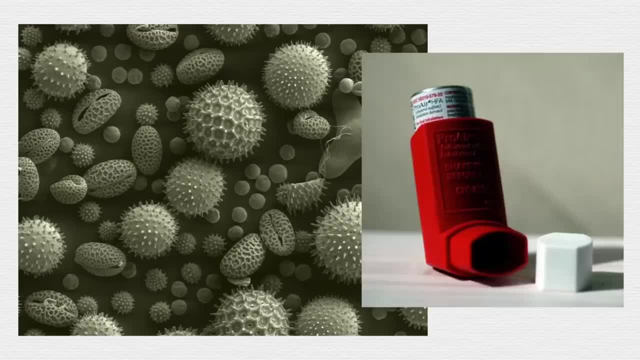 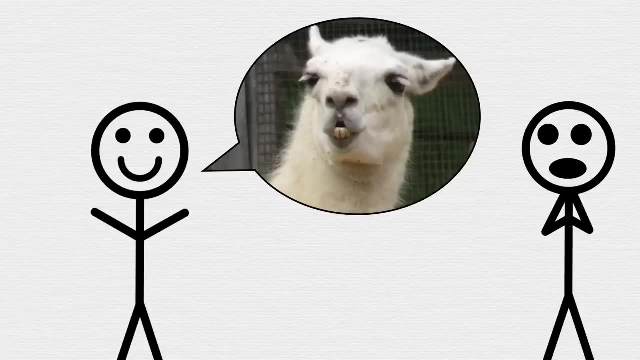 allergies and asthma cases are nocebic and thus able to be spread in the same way. To be clear, if someone's having an asthma attack, that's not the time to tell them. you know they're being a drama llama because you watched an internet video about the nocebo effect. They're really having an.